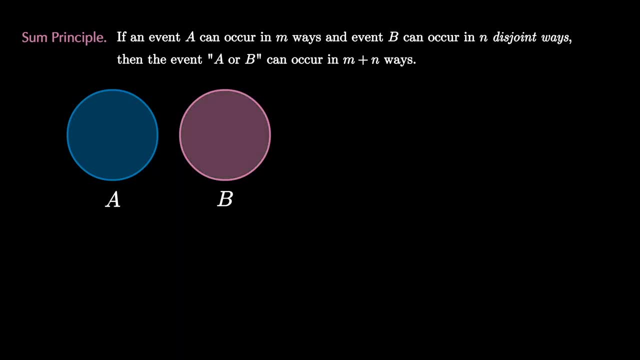 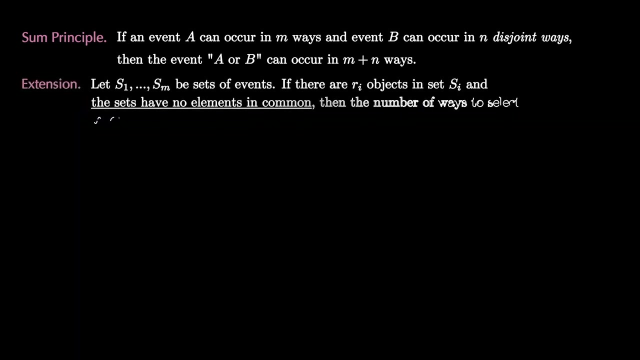 translation of the sum principle for sets, by noting that if we have the sets A and B and they do not overlap, then we can determine the cardinality of their union just by adding the cardinalities of the separate sets. as seen here, The sum principle can be generalized to more sets. So if we have sets S1 up to SM, 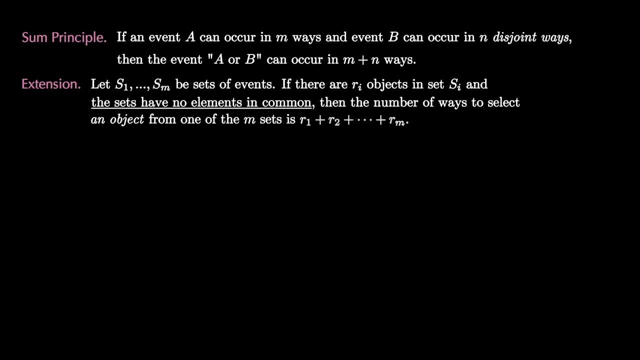 and there are RI objects in each set- SI- then if the sets have no elements in common, the number of ways to select a single object from one of the M sets is given by the sum of the total numbers of elements in the sets, which is R1 plus R2, all the way up to adding RM. 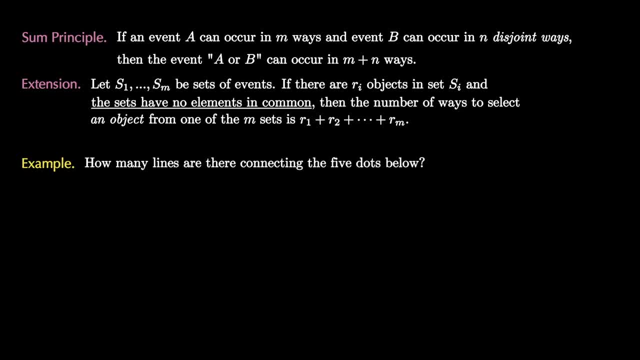 Let's see how this works. We can see that the sum principle can be generalized to more sets, as seen here. Let's see an example of this. How many lines are there connecting the five dots shown below here? If you watch carefully, it gives an idea about how to think about this. 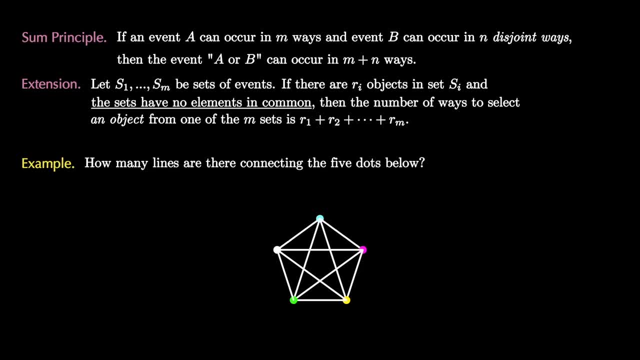 problem from the perspective of the sum principle. We can decompose the lines into four disjoint sets. The first set is the collection of lines that are connected to the blue dot. The second set are the lines connected to the pink dot but not the blue dot. The third set are the ones 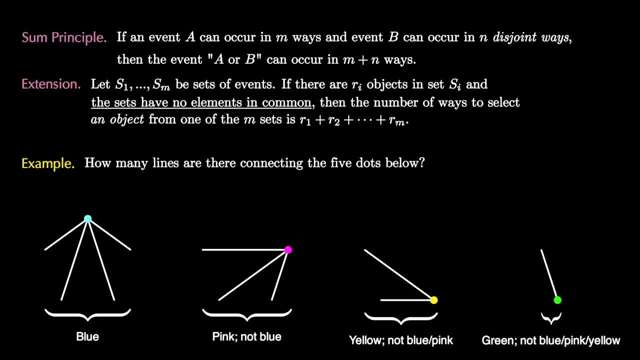 connected to the yellow dot but not the blue dot. The fourth set is the collection of lines that are connected to the blue dot but not the blue or pink dot. And the last set is the one connected to the green but not the other three colors. So the total number of lines by the sum. 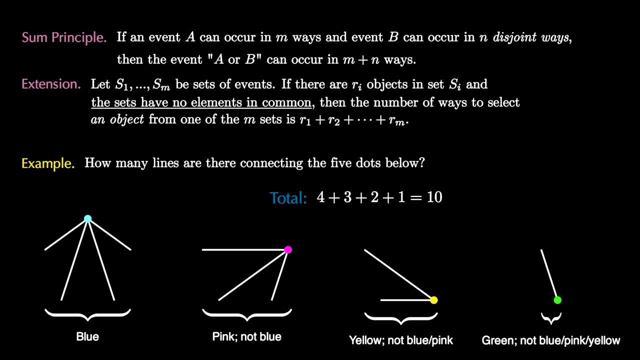 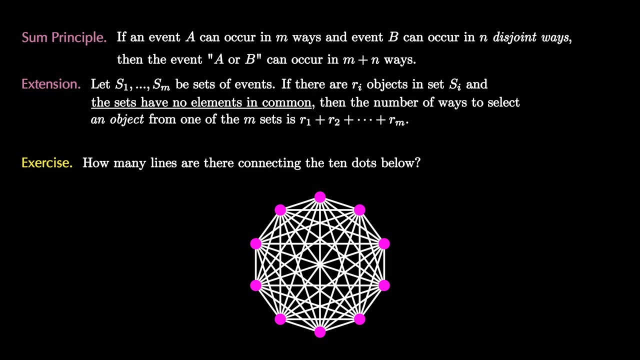 principle is 4 plus 3 plus 2 plus 1, which is 10.. Have another go at this yourself, but this time let's figure out how many lines there are connecting the 10 dots in the diagram below. If you watch carefully about how this diagram is built, you might be able to see the sum principle. 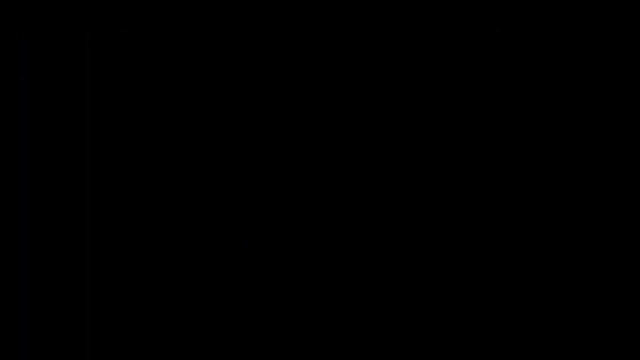 in action. The second important counting technique is the product principle. The product principle states that if event A can occur in m ways and each possibility for A allows for event B to happen in exactly n ways, then the event A and B can occur in m times n ways We can. 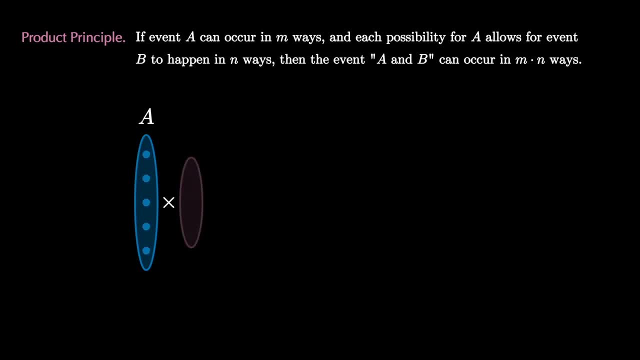 think of this as a direct translation of the formula for the cross product from set theory. corresponds to an ordered pair of something from a followed by something in b. The formula for the cross product can be determined by taking the set a and putting a copy of b on top of each element. 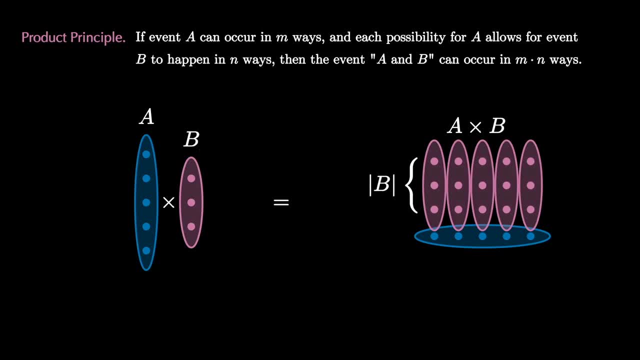 in the set a. Then we can pair each element from a with a corresponding element from b. What we are left with is a grid of size: cardinality of a by the cardinality of b. The resulting interpretation is that the cardinality of the cross product a times b. 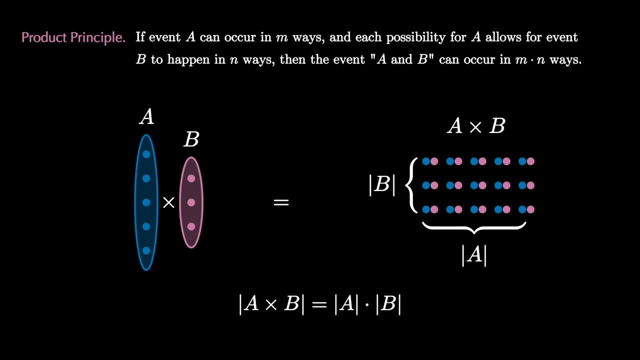 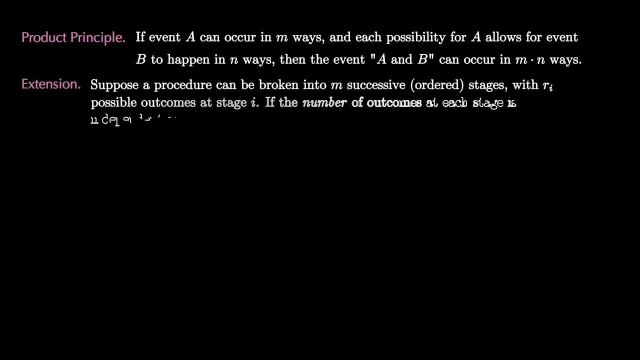 is equal to the product of the cardinalities of a and b. The product principle can be extended to multiple sets. So suppose a procedure can be broken into m successive ordered stages with ri possible outcomes at stage i, If the number of outcomes at each stage is independent of the number of choices in previous stages and the outcomes are. 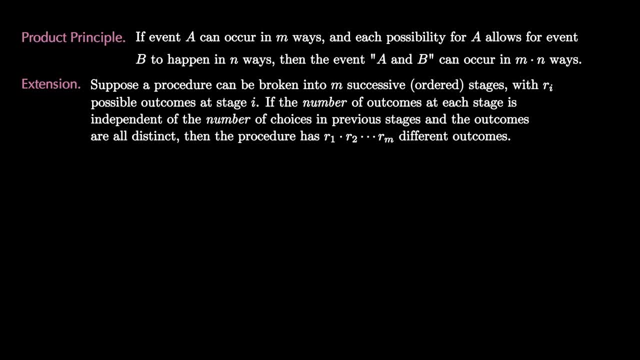 distinct, then the procedure has the product r1 times r2 up to rm different outcomes. Let's work out a straightforward example. How many strings can you create by rearranging the letters in the word math? Well, one thing we can do is that we can literally list them all out. 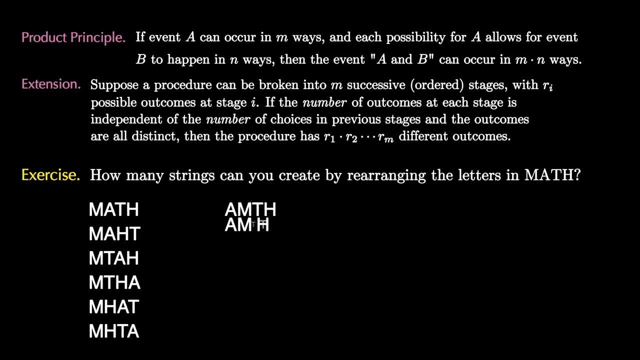 All we have to do is be careful to make sure that we haven't repeated any of the words or strings that we've seen before. What we end up with is this list. but notice, in this list we've already done something interesting. We've organized them by the first letter, m, a, t and h, And then within each column. 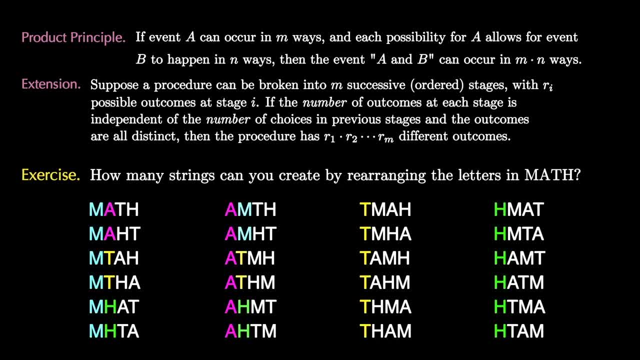 where the first letter is fixed, we notice that with the number of second letters that can appear is each time, And then the number of third letters is the same and the number of fourth letters is the same. Our enumeration shown here gives us an idea of how to understand the product principle. 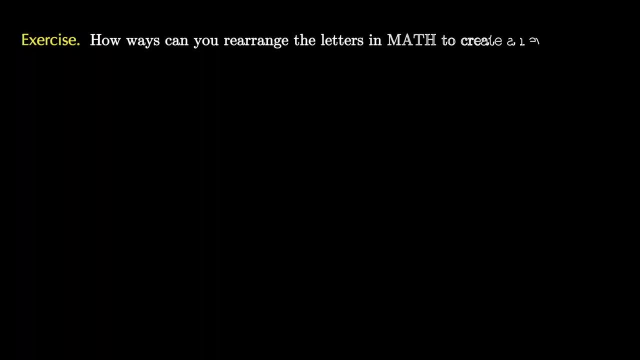 We will organize the strings in a chain of order, Because that way we can create the idea of a property: soldiers. In this way we can always understand when something is installing. Now it has gone a long way. the strings in a tree diagram. The first level contains the first letter of the string, The. 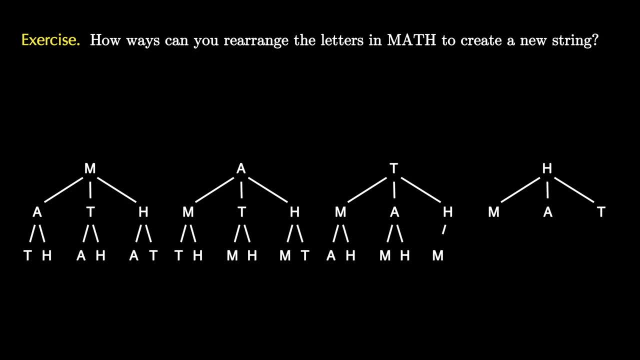 second level contains the second letter of the string. The third level contains the third letter of a string, And the fourth level contains the fourth letter of the string. So the strings correspond to paths from the top to the bottom. Now we see that we can do our counting using this. 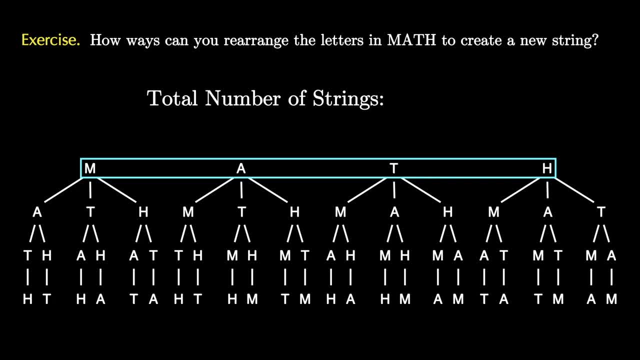 tree diagram. So the total number of such strings comes from a path in the tree. We have four choices for the first letter, And then, no matter what letter we choose, there are three choices for the second letter, And no matter what pair of letters we choose, first there are two choices. 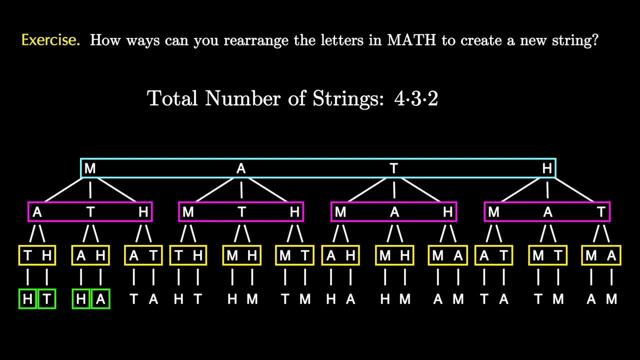 for the third letter, And no matter what triple of letters we pick, there's one choice of letter for the fourth letter. Since the number of choices is independent at each stage, we can multiply the numbers together to get that the total number of strings is 4 times 3 times 2 times 1, which is 24.. 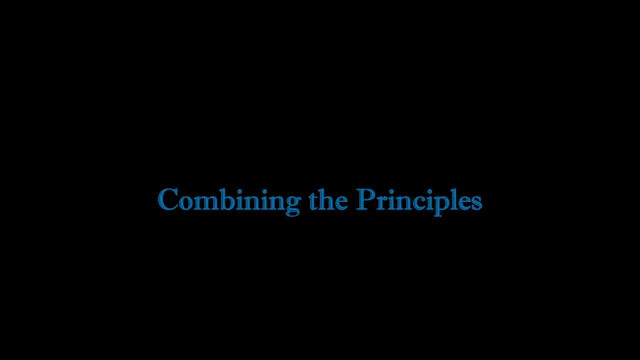 Even though the sum and product principles may seem kind of elementary, they can actually be utilized to do some very powerful counting. The idea is that we can provide complex counting arguments by merging the two principles. We may describe the objects so they can be built in. 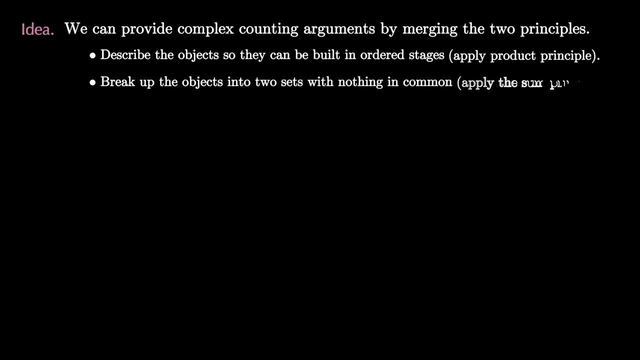 ordered stages and apply the product principle. We can break the objects into two sets with nothing in common and apply the sum principle, And then, once we're trying to figure out the number of things that can happen at a stage or in a disjoint set, we may have to repeat the process. 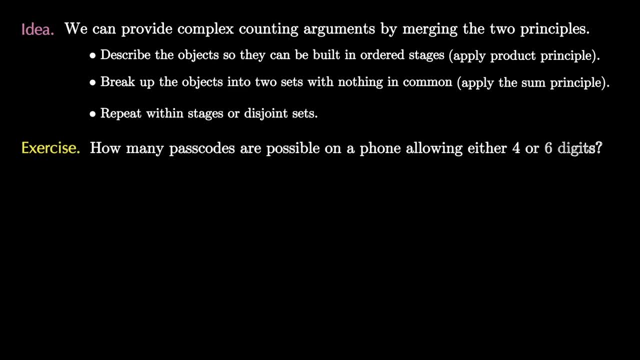 Let's try this out with an exercise. How many passcodes are possible on a phone that allows either four or six digit passcodes? Pause the video and try this first, before our discussion. The word OR already tells us what to do. It tells us to break it into two disjoint situations, where 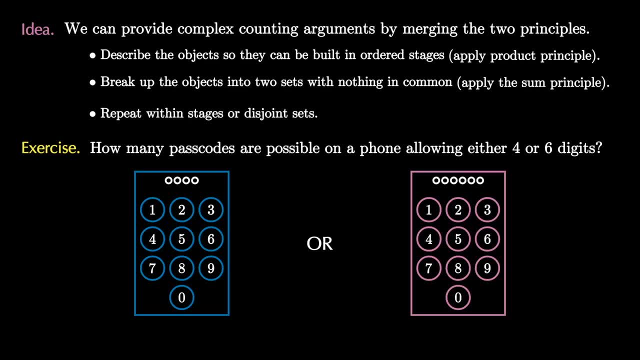 we either choose a four digit passcode or we choose a six digit passcode. These cannot overlap. Now, if we focus only on the four digit passcodes, we see that we have free choice for each of the digits. So we can simply press some digit, then a second digit, then a third digit, then a fourth. 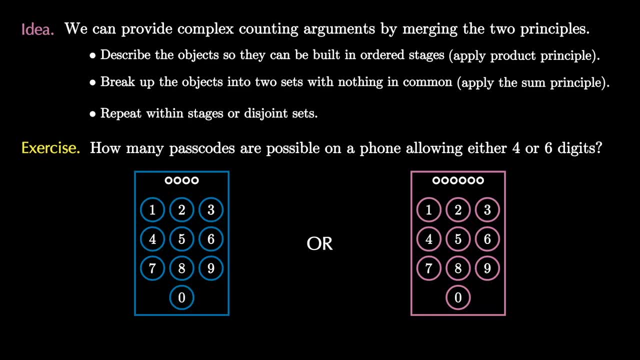 digit. This means, since we have 10 choices for each digit, we can apply the product principle And we see that there are 10 times 10 times 10 times 10 total such passcodes. The same analysis works on the six digit passcodes. We get a six digit passcode by just choosing the first digit. 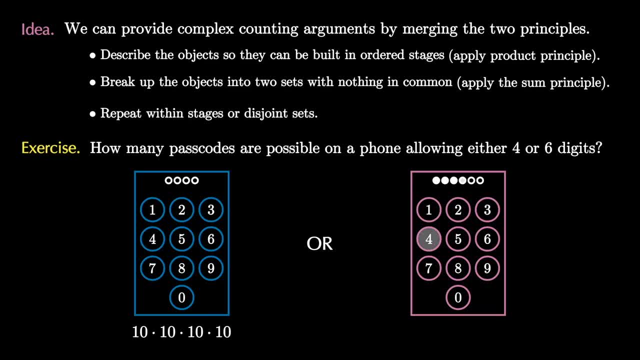 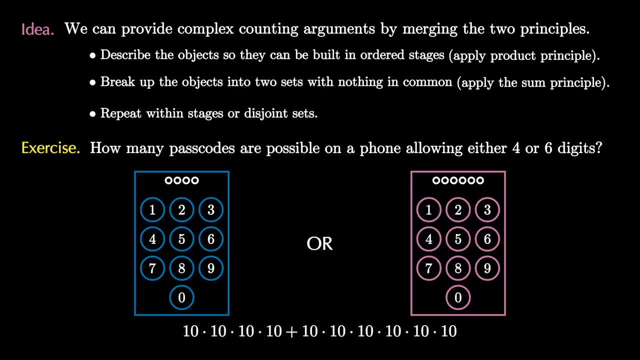 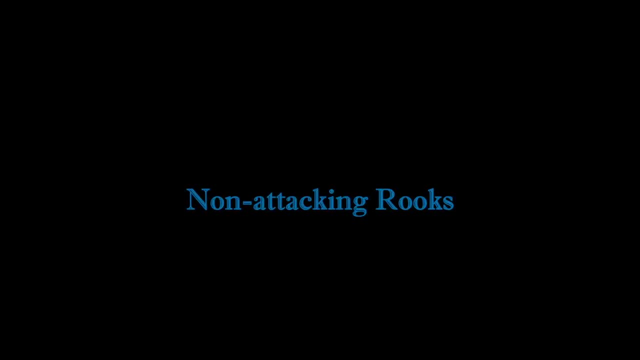 such passcodes Using the sum principle, then we get the total number of passcodes as 10 to the fourth plus 10 to the sixth. We have applied both the sum principle and the product principle to determine the total number of possible passcodes on such a phone. Let's revisit our question that. 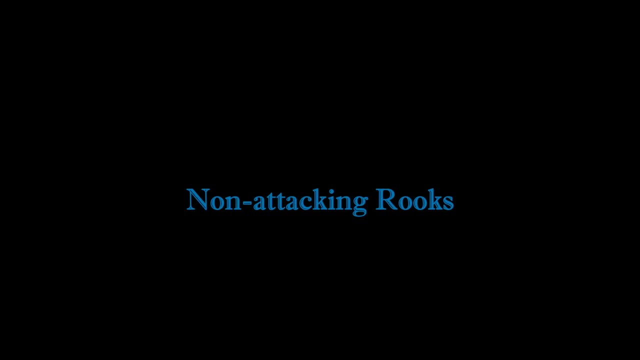 started the video off about non-attacking rooks on a chessboard, Recall that we wanted to know how many ways we can place eight rooks on an 8x8 chessboard in such a way that no rook can attack another. We can answer this question by applying the 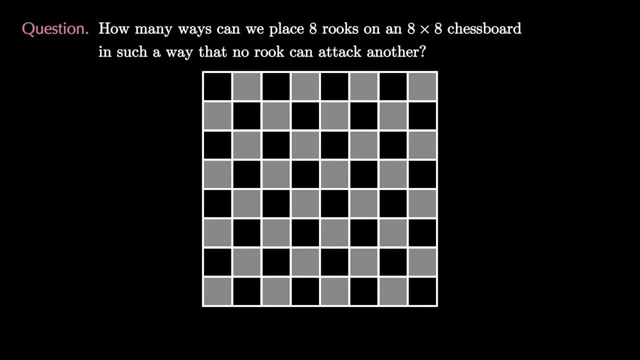 product principle by noting that each column must contain one and only one rook. So we can go column by column as our ordered stages. In the first column we have eight choices where we can place the rook, But once we place a rook we remove that column and its row. so that now, in the second, 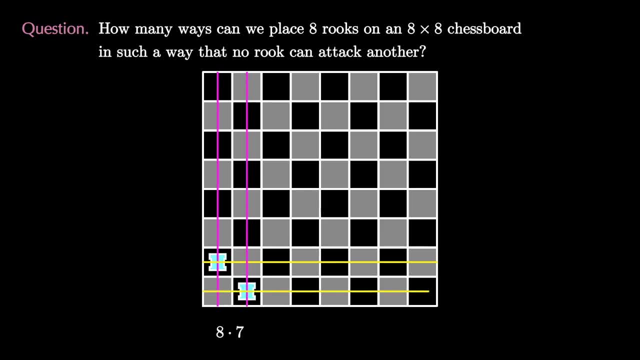 column we have only seven choices for where to place the rook. Again, it removes the column and the row. So in the third column there are only six choices for where to place the rook. It removes the column and the row. So then in the fourth column there are five choices for where to put. 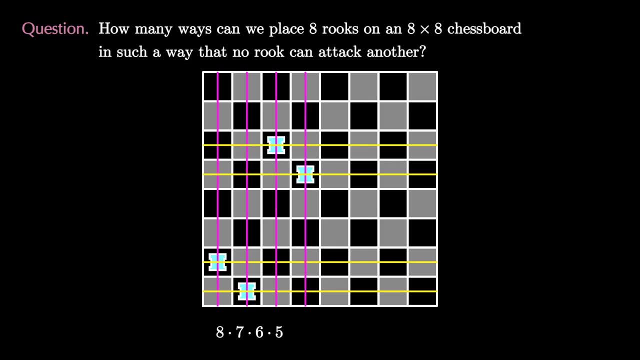 the rook. But once we do that, we remove that column and that row. Now there are only four choices for the next rook. Once we place it, we remove the column and the row. So the next rook has only three possible choices for where we can place it. Once we place it, we remove the column. 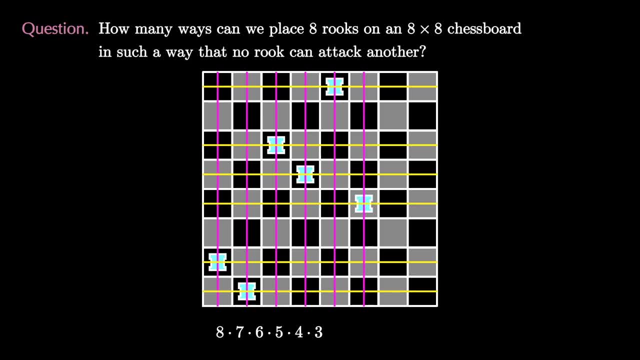 that rook, we remove the column and the row, So the second to last rook has only two choices. And once we place that rook, we remove the second to last column and that row. Therefore, there's only one place left to place the final rook. Even though we showed just a single example,